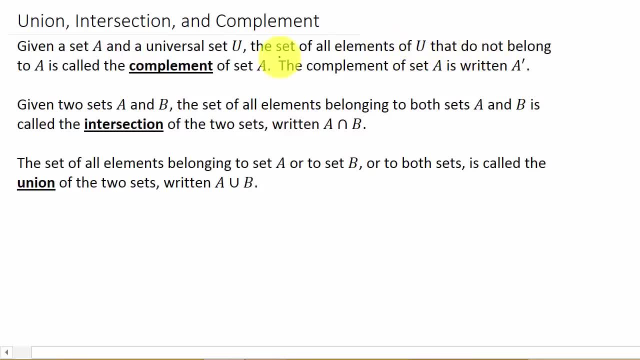 of all elements of U that do not belong to A is called the complement of set A, And the way we write it is with this, A prime here. okay? So basically, if you have a universal set U and you have a set A and A has some elements in it, well, every element that is not in this one in A. 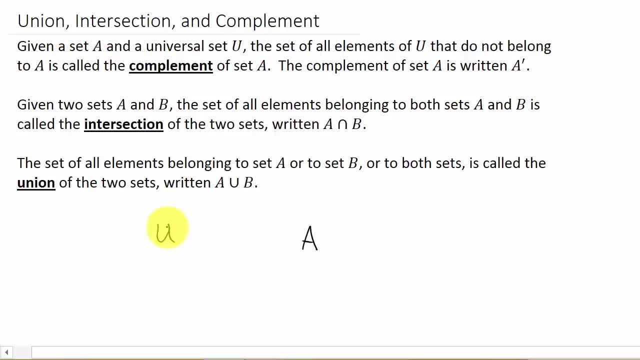 but is in the universal set. that's the complement of a, and I'm gonna do some examples, so I've got about eight examples to work. all right, so, and then we have the intersection. so, given two sets, a and B, the set- all of all elements that belong to both sets, sets a and B- is: 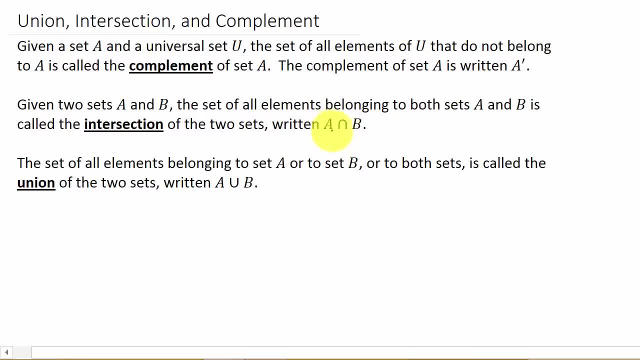 called the intersection of the two sets, and this is how we write it: a intersect B and then this and then the set of all elements belonging to set a or to set B or to both sets. it's called the u-get of the two sets and we write it like: 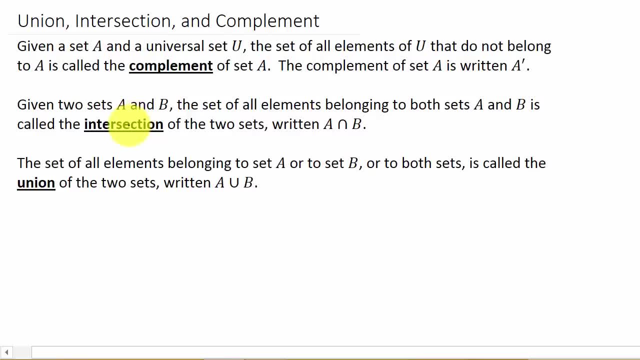 this a union B. so intersection is basically: if you want to find the intersection of two sets, it's the elements they have in common and the union of two sets. so if you have two sets and you want the union, it's just every element that's in both sets combined into one set. okay, so let's go. 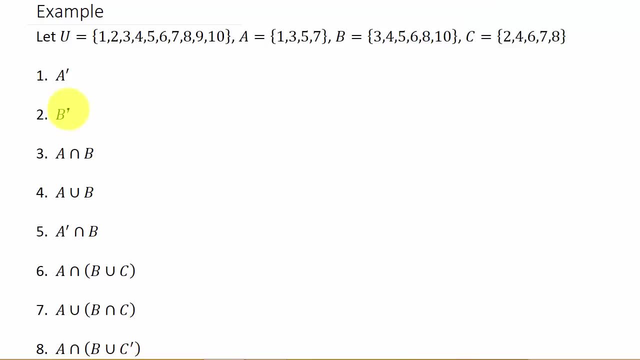 ahead and look at the intersection of two sets and the set of all elements and get started on the example. so you can see I've got about. I've got eight examples to work, all right, so let's look at this. so we want to find the complement of a. well, here we have the universal set, so the universal set. 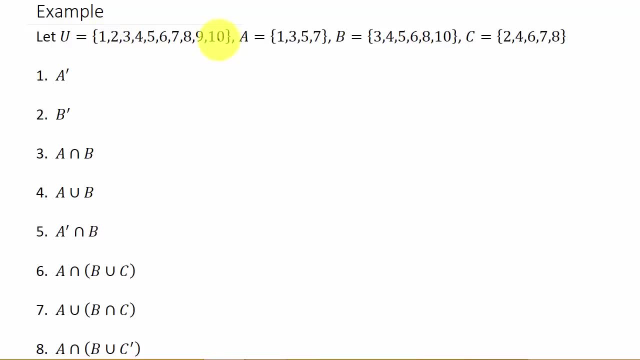 contains of: contains the set of numbers, of the numbers one through ten, here set a, one, three, five, seven, set B and set C. all right, so we want the complement of a. so the complement, remember the complement of a, is all of the elements that are not in set a but are in the universal set. so you see how set a 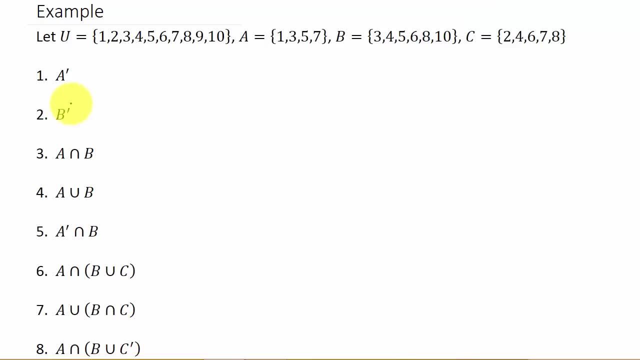 ahead set B or to both sets. it's called the union of the two sets and we write it and get started on the example. so you can see I've got about. I've got eight examples to work, all right, so let's look at this. so we want to find the 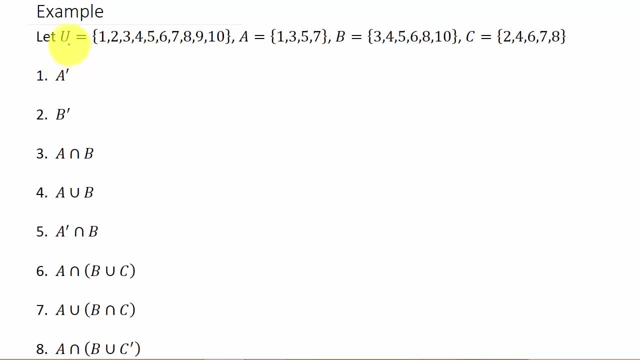 complement of a. well, here we have the universal set. so the universal set contains of, contains the set of numbers, of the numbers 1 through 10, here set a, 1, 3, 5, 7, set B and set C. all right, so we want the complement of a, so the 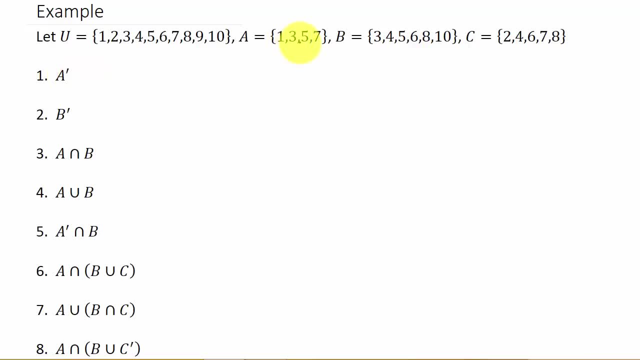 complement. remember, the complement of a is all of the elements that are not in set a but are in the universal set. so you see how set a contains the numbers 1, 3, 5 and 7. okay, so if you see that, see 1, 3. 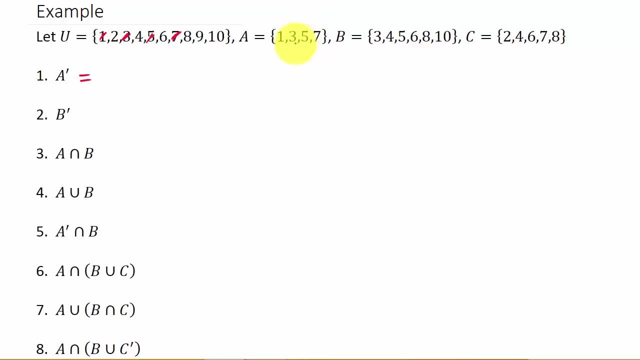 7, 5 and 7. those are the elements that are in set a. well, which elements are not in set a but are in the universal set? you see that's 2, 4, 6, 8, 9 and 10. so the complement of a would be 2, 4, 6, 8, 9 and 10. and there's your answer. okay, all right. 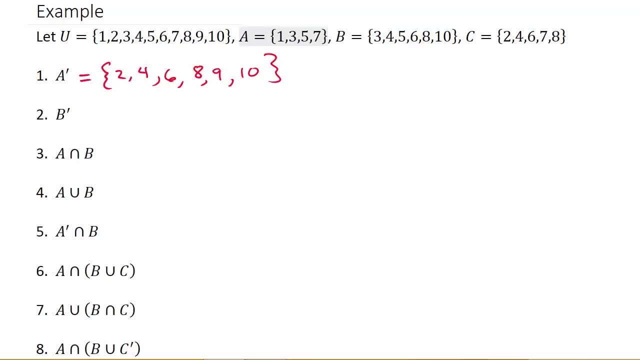 so let's look at a. let's look at the next one, the complement of B. okay, so the complement of B is everything that's in the universal set that's not in set B. so let's see what's in B. so we've got what? 3, 4, 5, 6. so 3, 4, 5. 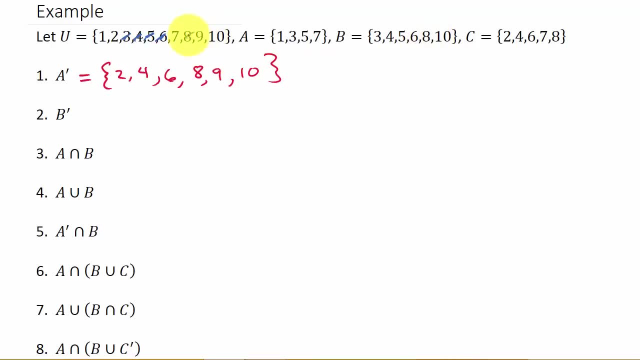 six, eight and ten, eight and ten. okay, so this would be what? one, two, one, two, let's see seven and nine, and so that's the complement of B. all right, now let's look at a intersect B. all right, so a intersect B. we look at sets a and we look at sets B, set a and. 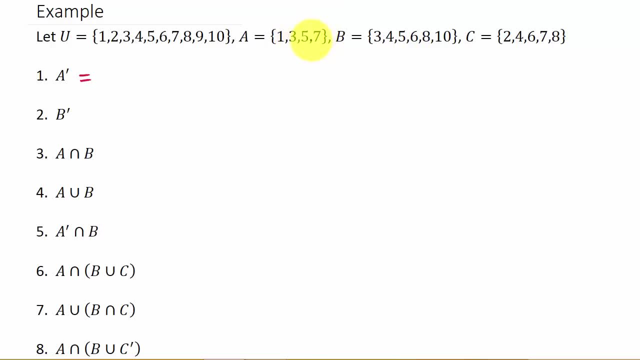 contains the numbers one, three, five and seven. okay, so, if you see that, see one, three, seven and seven. those are the elements that are in set a. well, which elements are not in set a but are in the universal set? well, you see, that's two, four, six, eight. 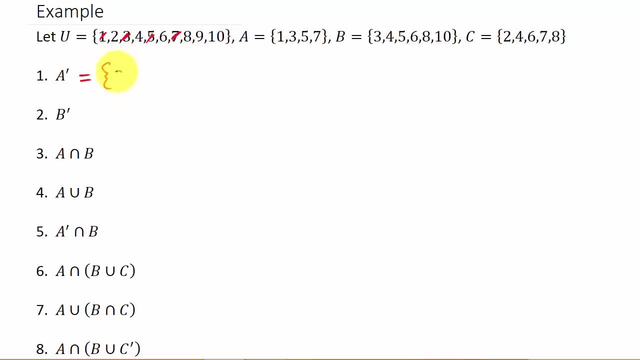 nine and ten. so the complement of a would be two, four, six, eight, nine and ten, and there's your answer. okay, all right. so let's look at a. let's look at the next one, the complement of B. okay, so the complement of B is everything that's in the universal set. 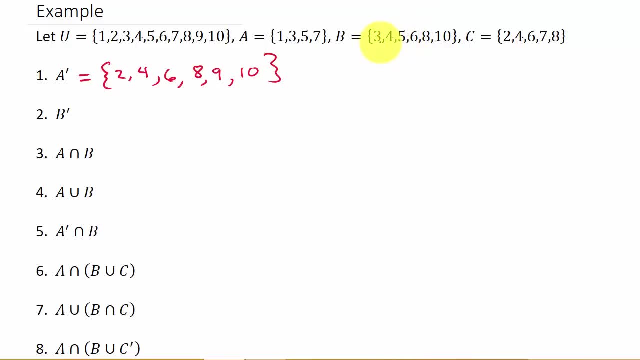 that's not in set B, so let's see what's in B. so we've got what: three, four, five, six. so three, four, five, six, eight and ten, eight and ten. okay, so this would be what: one, two, one, two, and let's see seven and nine, and so that's the complement of B. all right now. 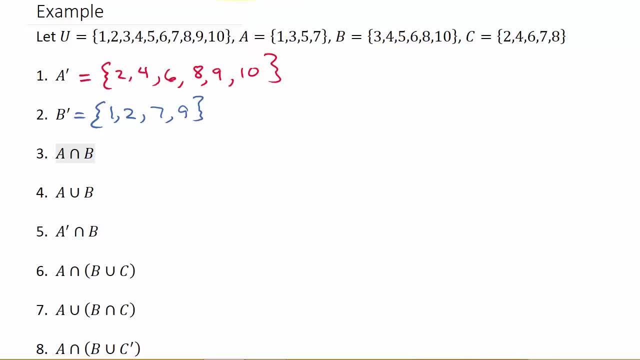 let's look at a intersect B. all right, so a intersect B. we look at sets a and we look at sets B. set a and B. now we want to know: what do these sets have in common? well, let's see. well, B does not have a one. so we look at the three. well, 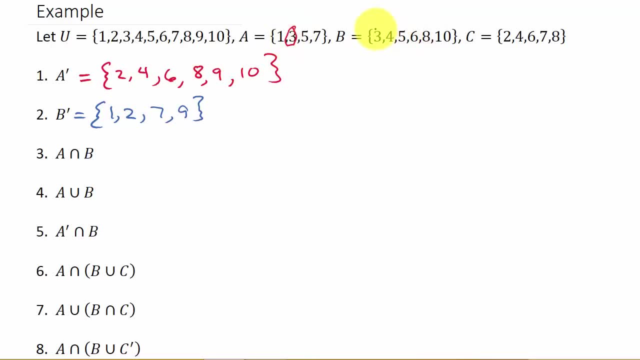 B has a three. so there's one element that they have in common: three. let's see five. yep, there's a five here and a five here, and then seven. well, B doesn't have a seven. so the only elements they have in common is three and five. so this: 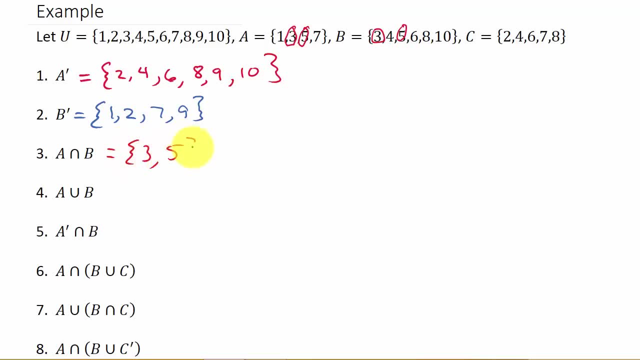 would be three and five. all right, and then a union B. well, all that is, let me do this, all right. so a union B, that's all of the elements from sets a and B combined into one set. so we've got a one, a three and see B has a three, but we only write it. 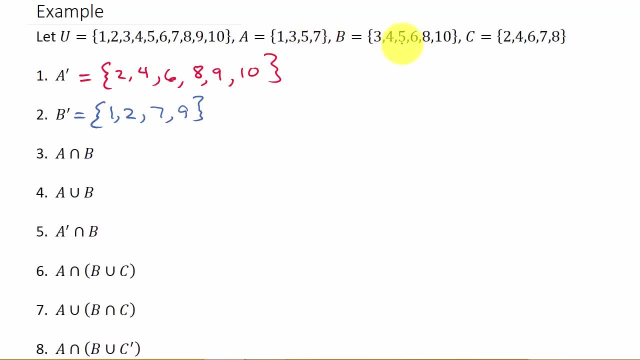 B. now we want to know: what do these sets have in common? well, let's see. well, B does not have a 1, so we look at the 3. well, B has a 3, so there's one element that they have in common. 3- let's see. 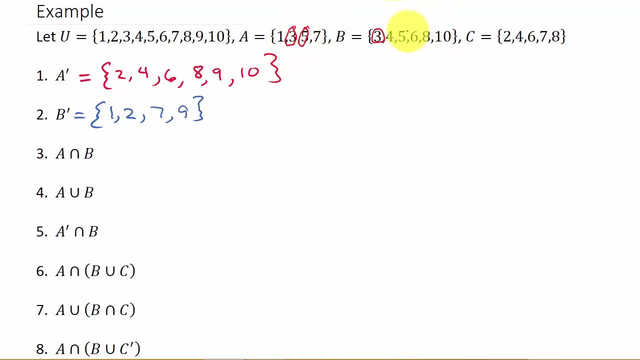 5. yep, there's a 5 here and a 5 here, and then 7. well, B doesn't have a 7, so the only elements they have in common is 3 and 5. so this would be 3, 5, right, and then a union B. well, all that is, I mean. 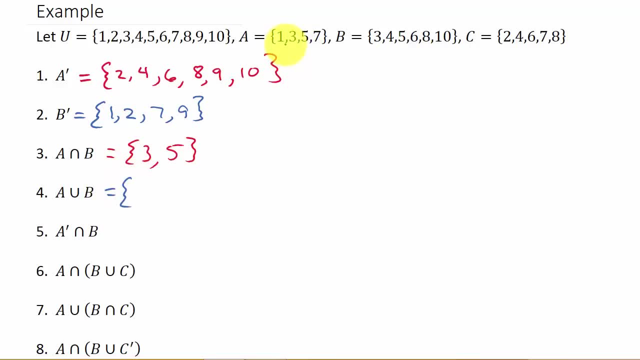 all right, so a union B, that's all of the elements from sets a and B combined into one set. so we've got a 1, a 3 and see B has a 3. but we only write it one time, you don't write it twice. okay, so 1- 3. 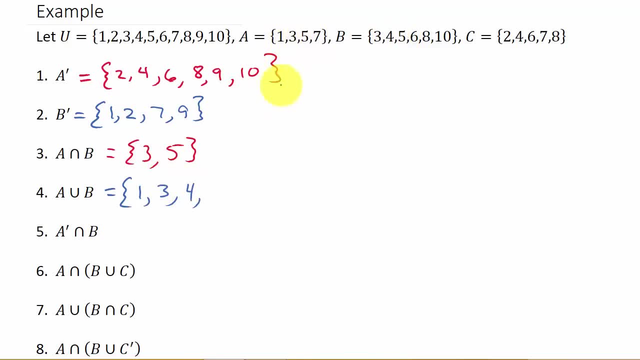 and then let's say we got a 4 here and then a 5, and then let's see there's a 6- just try to keep the numbers in order- 6, and then we've got 7, 8 and 10, and so there's a union B. okay, there's a union B. 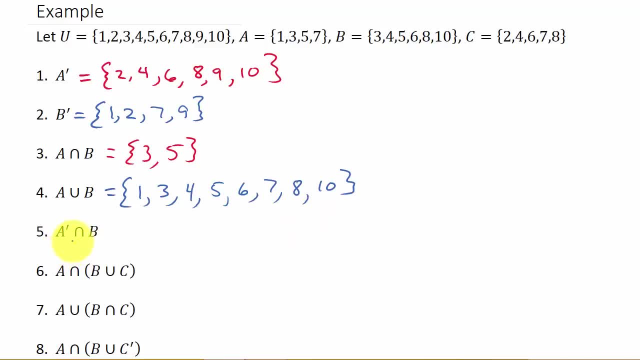 all right. now let's look at this one. we've got the complement of a intersect B, all right, so let me go ahead. I'm going to erase this so I have some room to work, because we're going to have to. we'll have to do a little more work with these, all right? 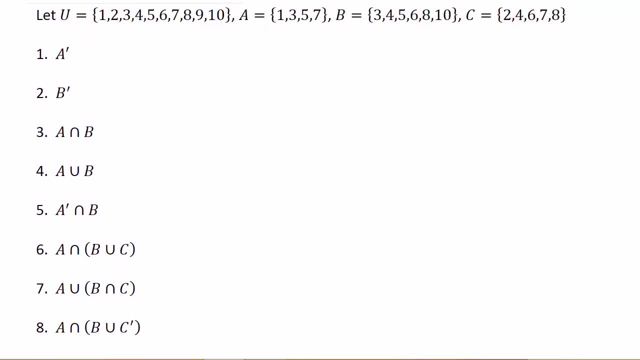 I'm going to bring this up just a little bit, all right, so what we want to do here is: I need the complement of a and B, okay, so I need to know what elements does a complement and B have in common? well, I don't have the complement of a. I know we had it right here, but I erased it. but let's go. 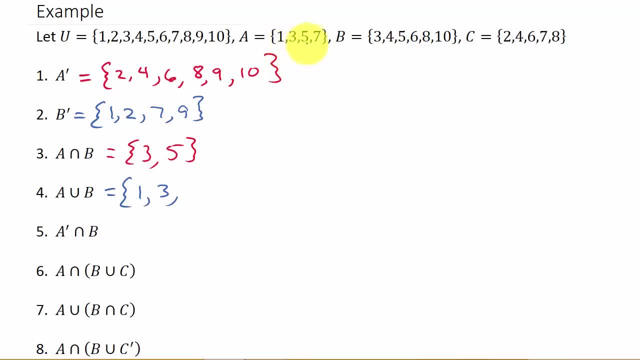 time you don't write it twice, okay, so one, three, and then let's say we got a four here and then a five, and then let's see there's a six- just try to keep the numbers in order- six, and then we've got seven, eight and ten, and so there's a. 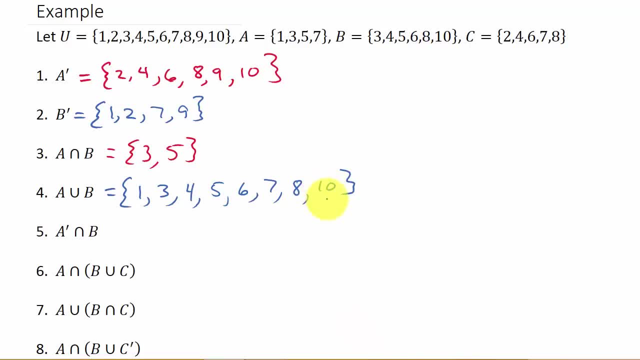 union B. okay, there's a union B, all right. now let's look at this one. we've got the complement of a intersect B, all right, so let me go ahead. I'm gonna erase this so I have some room to work, because we're gonna have to. I have to do a. 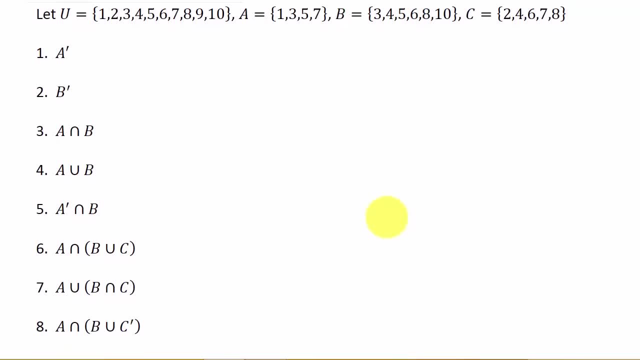 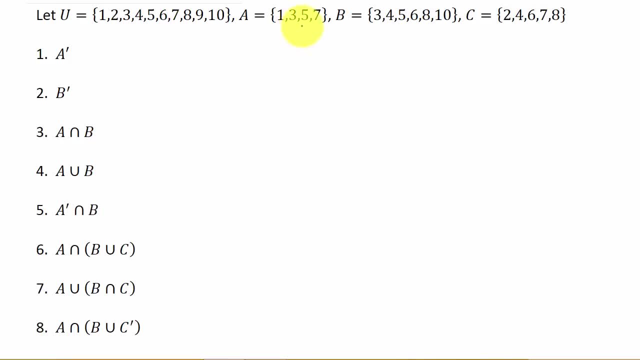 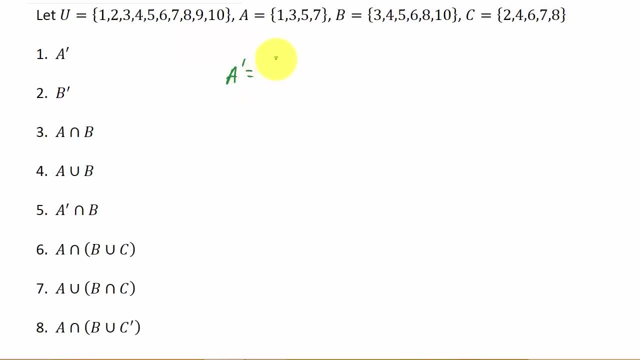 ahead and write it down. so the complement of a is equal to: so remember that's going to be what: two, four, six, eight, nine and ten. so there's the complement of a. make sure I've got everything. one, three, five, seven. one, three, five, seven. so, yeah, that looks right. all right, so now I want to know: what does a complement and B have in common? 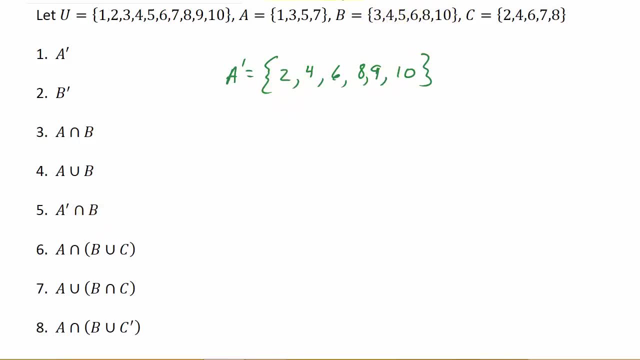 so here's a complement, here's a, B. well, let's underline the, the numbers they have in common. so let's see, they've got a four in common, okay, they've got a six in common, and they've got eight in common and they have a 10 in common, and so those are the values they have in common. so this: 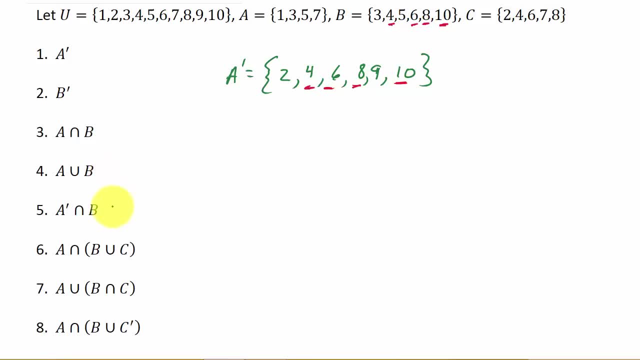 set would be. let's see that's going to be what: 4, 6, 8, 10, and so there's a complement intersect B, all right, all right. now let's look at the next one. we've got a intersect B- Union C. okay, a intersect B- Union C. so what we're going to do here? 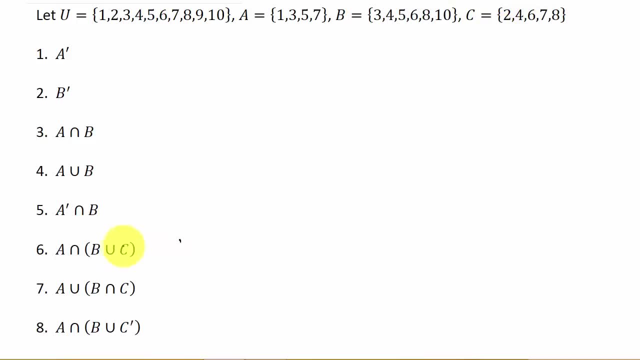 is notice that this is in parentheses, so we need to do this first and then do the intersection with a. okay, so first i need to find b, union c. okay, so that's all the elements from b and c combined into one set. that's what union means. so we've got a, two, three, four, five, six, seven, eight and ten. that's all the elements. 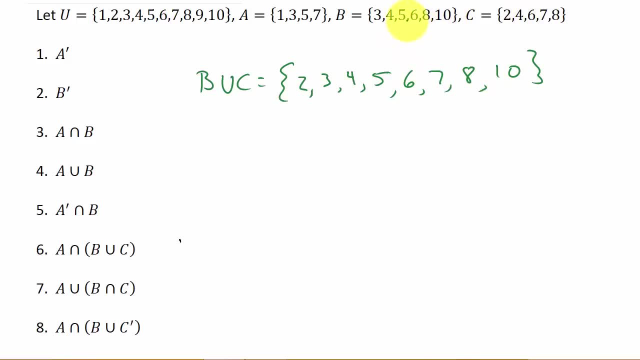 from both sets combined into one. and, yes, they both have a four, but you only write it once, don't write it two times, don't write it twice. okay, so there's b, union c. so what i want to do is i want to take this set here and intersect it with a, so i need to know what elements does this set and this set? 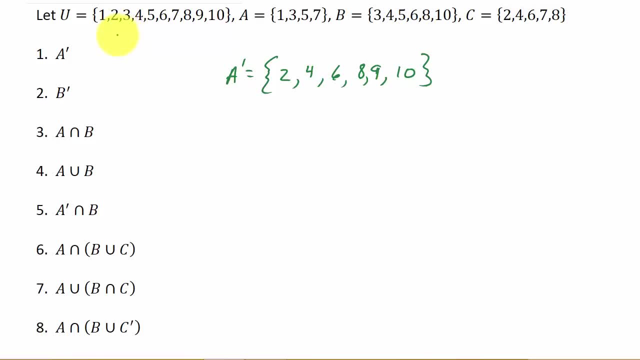 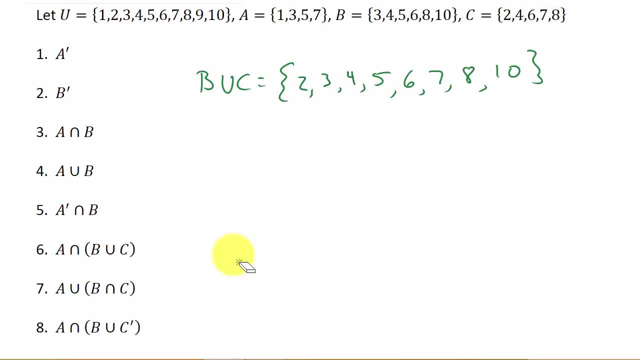 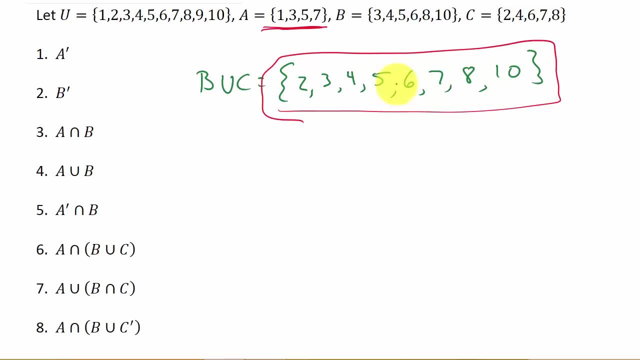 have in common, okay. so let's see. well, we can, let's let's underline what they have in common. that might make it a little easier. so let's see: well, they both have a three, uh, they both have a five and they both have a seven. okay, and so that would be the answer here. that would be three, five, seven. 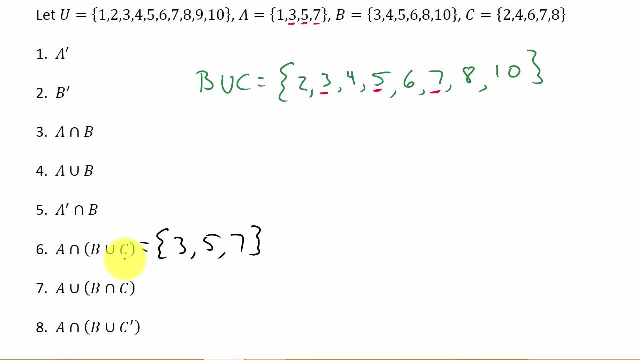 and there's a intersect b, union c. okay, all right, so let's look at the next one. all right, so we've got a union b and an intercept c. so once again, we need to do what's in the parentheses first. okay, so i need b intersect c. so remember: b intersect c. that's what these two sets have in common. okay, i'm finding. 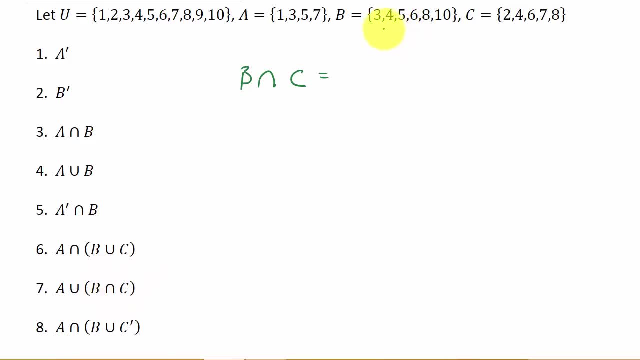 this first. so let's look, what does b and c have in common? well, let's say they both say they both have a four, They both have a 6, and they both have an 8, okay. So the intersection of B and C would be 4,, 6,, 8,, okay. 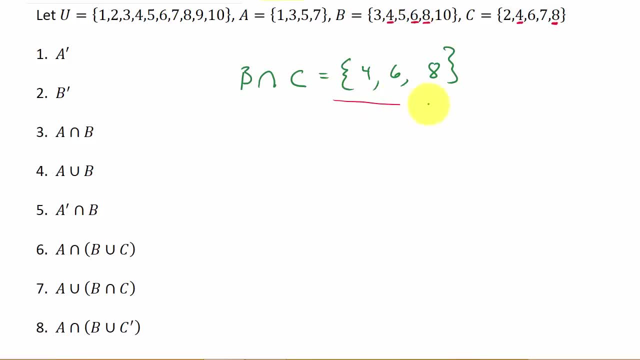 And now, what do I want to do? I want to do this set: union A, See A. union the B intersects C. all right, So remember, union, that's everything in this set, or everything in this set plus everything in this set, combined into one set. 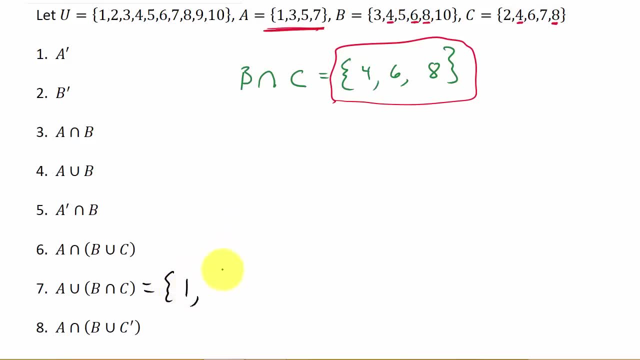 So that would be what: 1,, 3,, 4,, 5,, 6,, 7, and 8.. And you can see here nothing. they didn't have the same number in both sets, So it was. 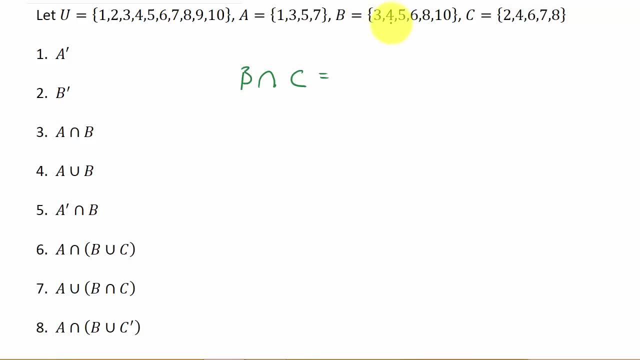 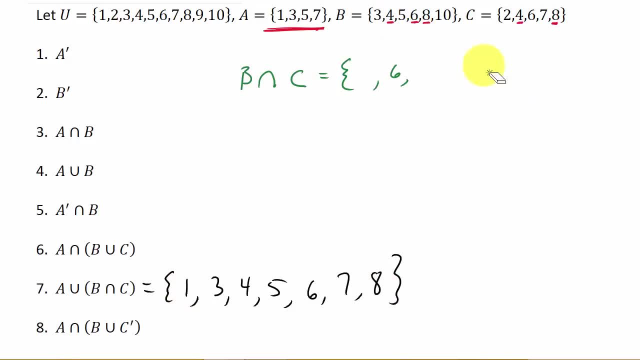 It was just every element. okay, All right, So let's take a look at the last one. All right, So I need A intersect B union C complement, okay, So once again, I need to find what's in this first, inside the parentheses. 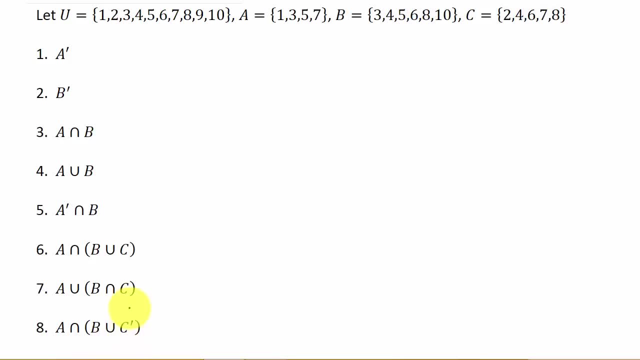 the union of B and the complement. I need to find the union of B and the complement inside the first set of B and C. So I need to find the union of B and the complement inside the first set of B and C. All right, 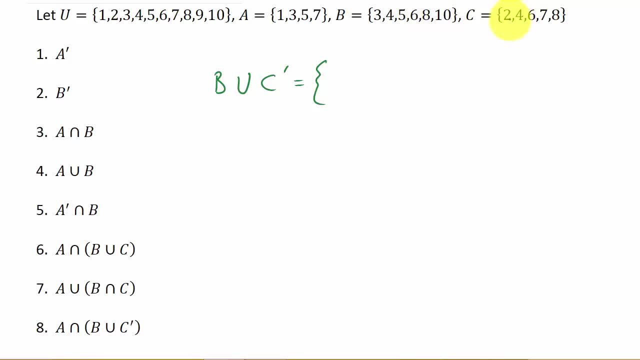 So let's see what we get. We get B union, C complement, all right, So remember, union, that's everything in this set and O and everything in C complement. Well, we don't have C complement. So look, we got to find that first, don't we? 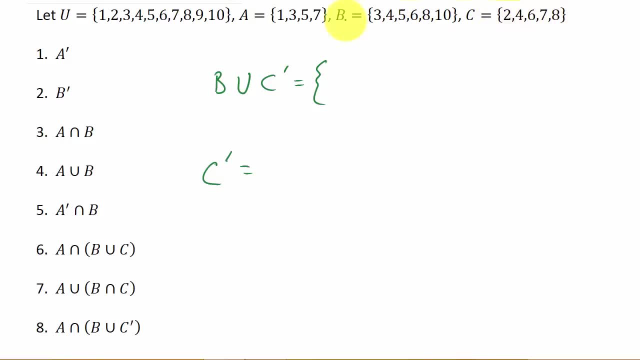 In set C. So let's see, Let's just cross out what's in set C. So that's the 2,, the 4,, the 6,, 7, and 8.. Those are the elements in C, But remember the complement. that's everything that's in here. that's not in here. 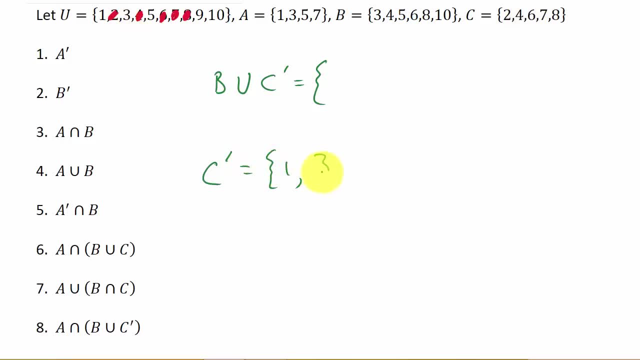 So that's going to be what: 1,, 3,, 5,, 9.. 9 and 10,. OK, So now I can do the intersection of B and C complement. I'm sorry, not the intersection, but the union. 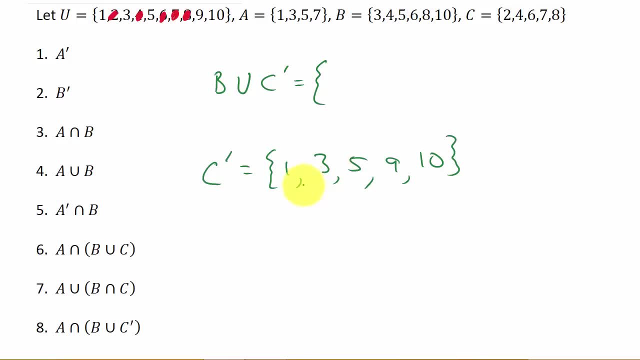 I can do the union of B and C complement. So the union is going to be everything in set B plus everything in C complement combined into one set. So let's see We've got what A 1,, a 3. 4. 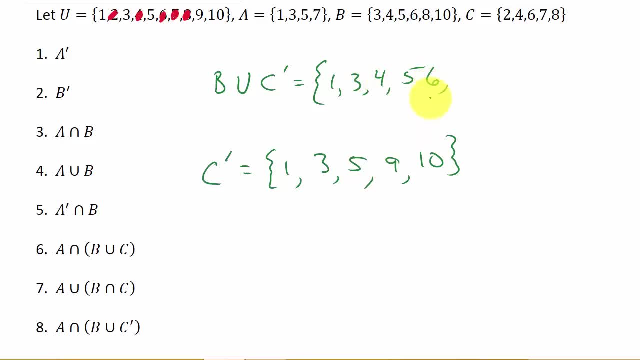 4, 5, 6.. 4, 5,, 6,, 8,, 9, and 10,. OK, That's everything from both sets combined into one set And, like I've said before, the 10 appears in both of them. 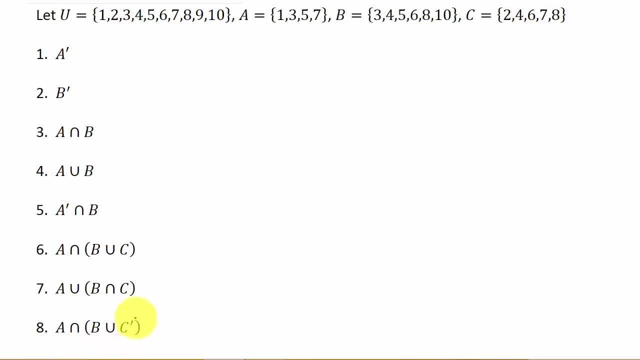